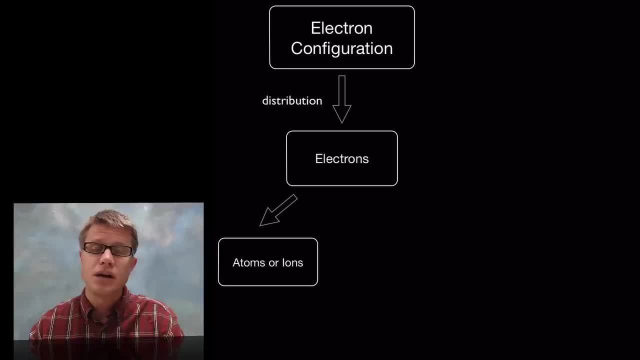 the distribution of electrons, So where the electrons are found In atoms or in ions, And so a good way to figure that out is to look at their ionization energy, Which is going to be the amount of energy it takes to pull an electron away, And so we can quantify. 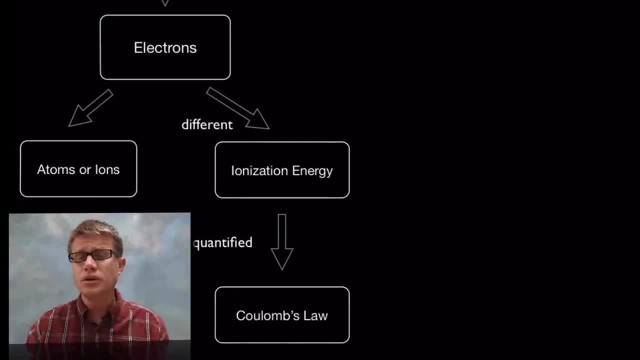 that by using Coulomb's law, And so what we can do is we can work our way out from the electrons on the inside to those on the outside, And when we're done, we have a pretty good picture of where all those electrons are. 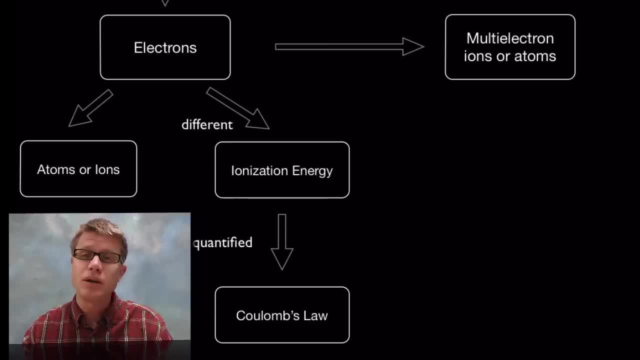 Because in most atoms they're going to be multi-electron, They have many electrons And what we'll find is there. they're going to be organized into shells, sub-shells and then orbitals, And all of those are going to have similar ionization energy And there's 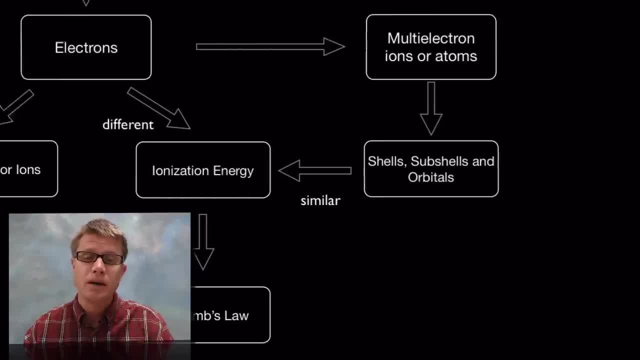 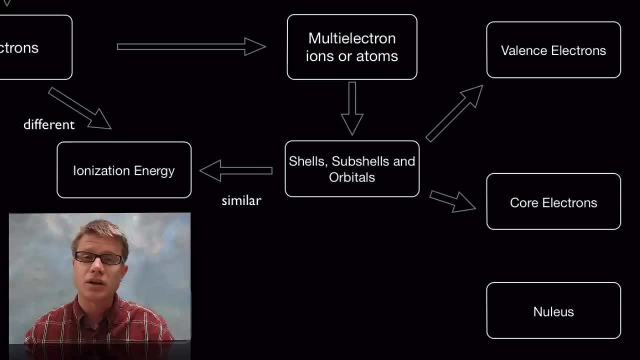 a chart on ionization energy. that's the most important one. Now, if we look at these orbitals and sub-shells, what we'll find is that the ones on the inside are going to be, or the inner electrons are going to be called core electrons, And the ones on the outside are. 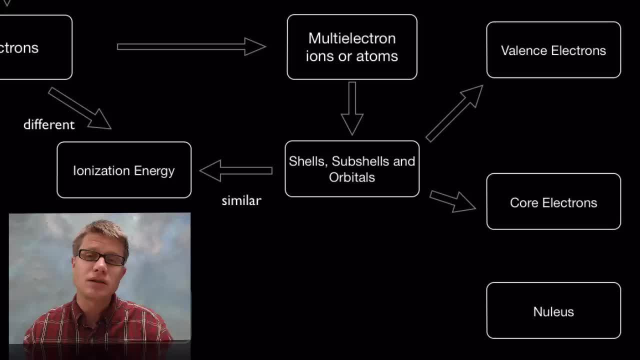 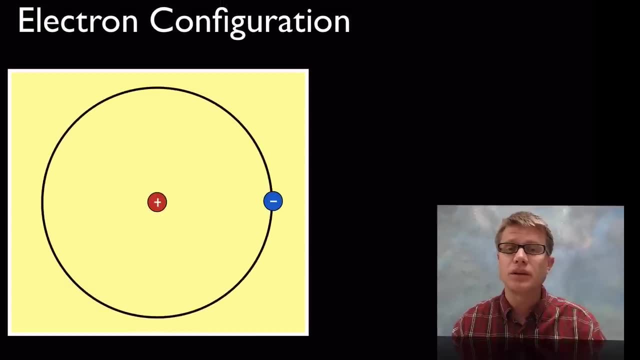 going to be called valence electrons. What we're going to find is that those on the inside, once they're filled, will actually shield the valence electrons from the power of the nucleus itself. And so let's look at the first and simplest of electrons. We've got hydrogen right here. One proton, One electron. 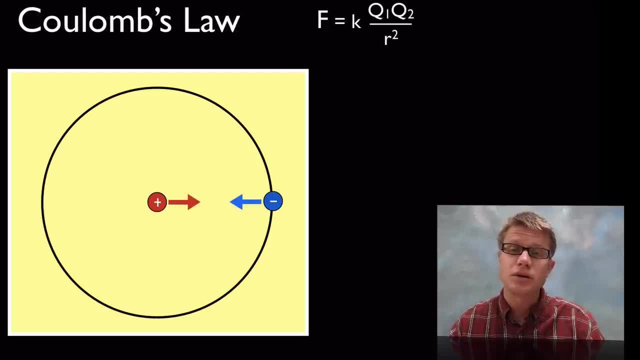 And so Coulomb's law allows us to quantify the force between the two, And so it basically comes down to the charges and then the distance between the charges. And so if we were to look at ionization energy, it's the amount of energy it takes to pull that electron away. 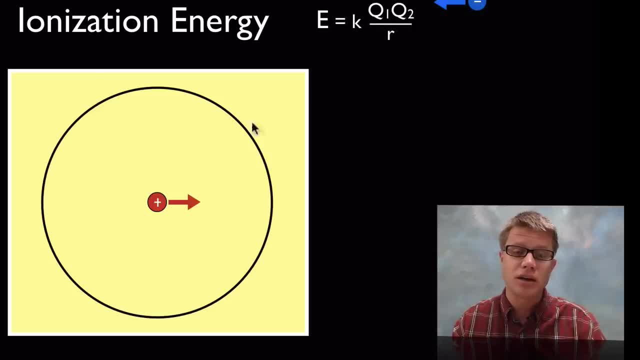 How do we figure it out? You're simply going to multiply the two charges. So let's say the proton has a positive charge, Let's call that plus 1.. And the electron has a negative charge, Let's call that negative 1.. And the only other thing we really need is the radius. 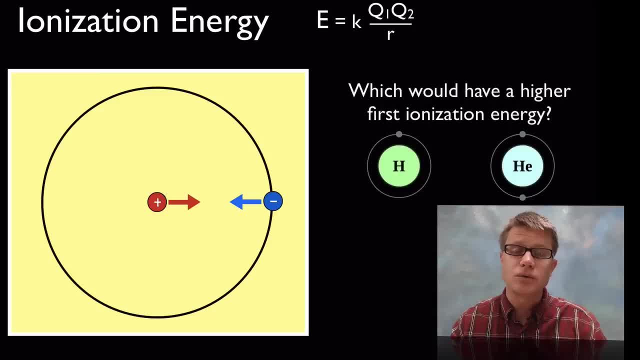 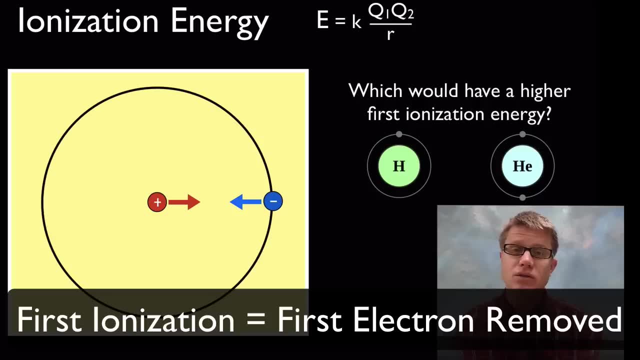 The distance between the two. And so let me ask you a quick question: Which do you think would have a higher ionization energy? Hydrogen, It's got one proton, one electron. Or helium, It's going to have two of each, And two neutrons as well. So make a guess And let me show. 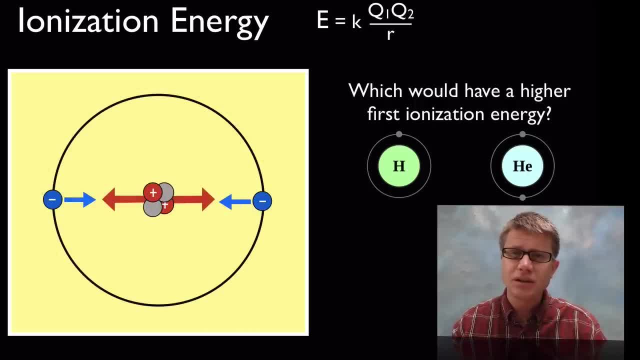 you what? Let's see what helium looks like. Helium, you can see it, just got a little bit smaller, And the reason why is, since it has two protons in the middle, there's going to be more pull Or there's going to be a larger energy of ionization in helium, And that's because there. 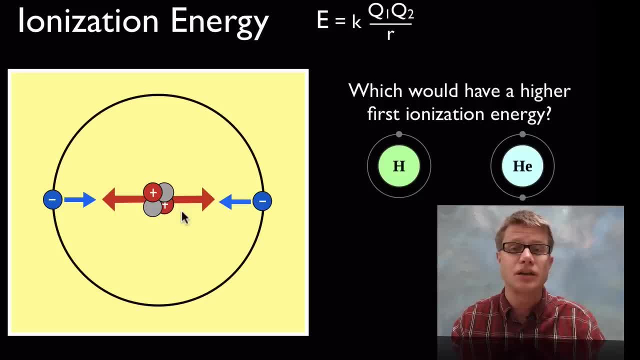 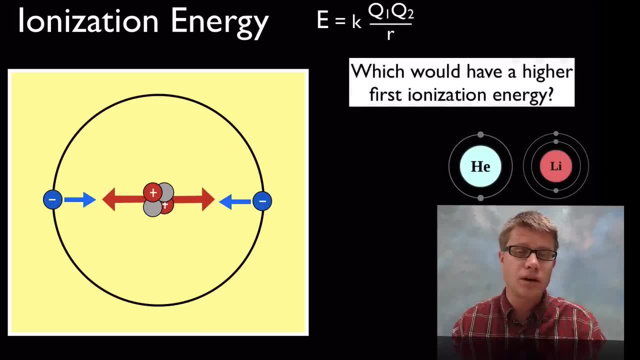 are a greater amount of positive charge on the inside. So we would say helium has a higher ionization energy. What about the next one? What if we were to compare helium then with lithium? What do you think happens to the ionization energy there? Well, you might immediately. 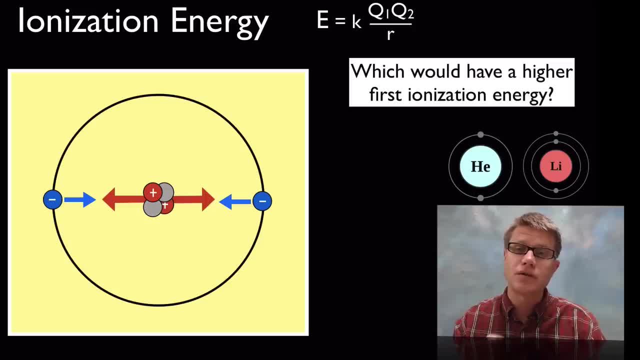 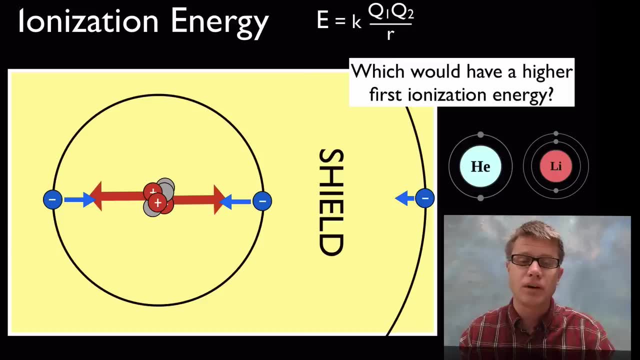 figure. But remember, the electrons are organized with only two electrons in that first shell And then when I learned it, it was going to be eight in that next sub-shell. And so if we look at that lithium, what we'll find is we've increased the number of protons. So 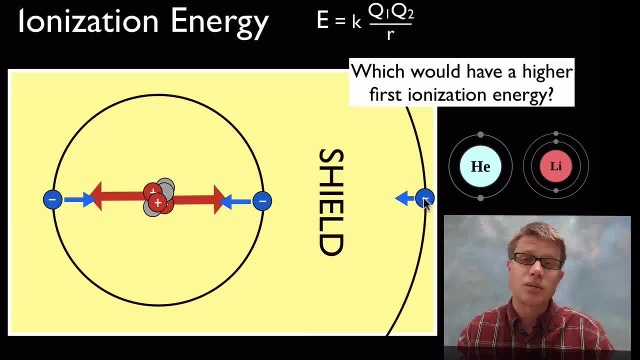 there's more of a charge here, But that electron is going to be in the next shell, And so, since it's in the next shell, it's shielded from the power of that protons- The protons in the nucleus itself- And so it's going to have a really small ionization energy here. Just 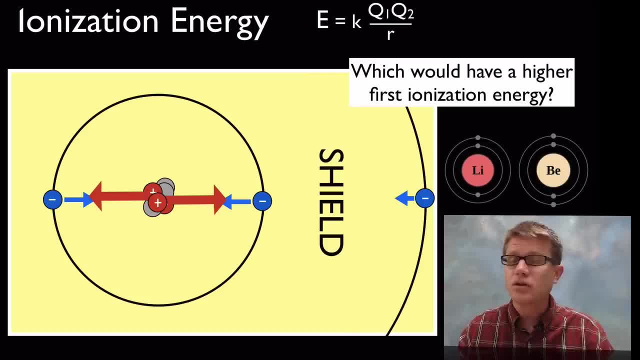 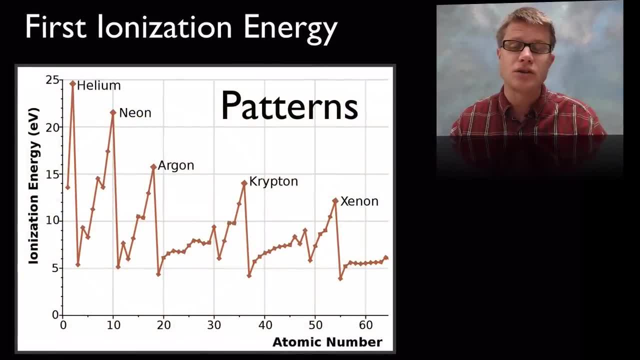 because of the shielding effect and the fact that we have another shell. And so what do you think about beryllium? Well, hold on to that and we'll take a look at the pattern. And so this is the chart that really allows you to understand what's going on with the 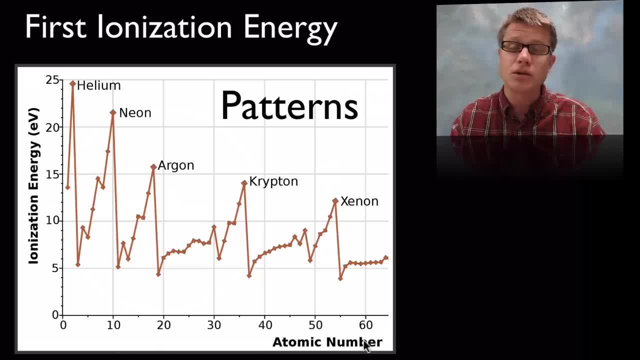 electrons, And so let me lay it out for you. We have atomic number across the bottom, So this would be hydrogen at one, Helium at two, All the way out, And then we're going to have ionization energy, which is the amount of energy it takes to pull that electron away. 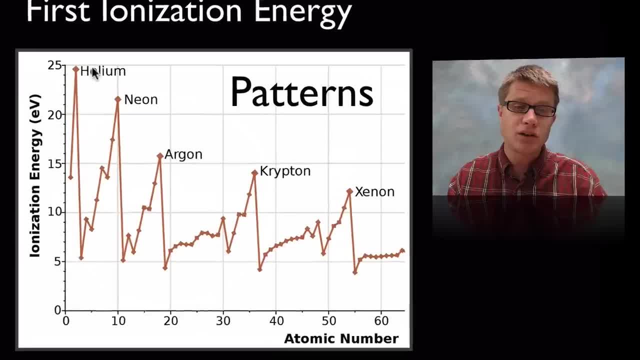 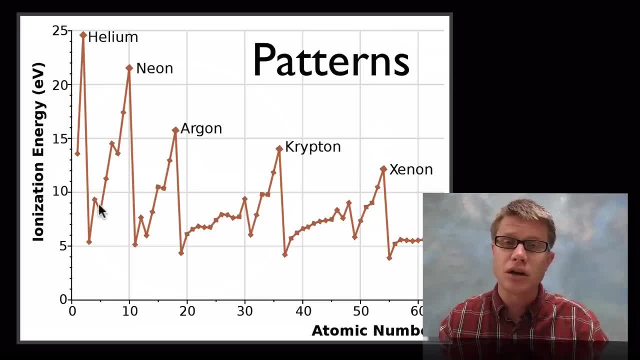 And what you can see are patterns immediately. And so these big spikes that you can see are with these noble gases, Those are going to be those different shells. You can see that they're broken down into sub-shells And then we're going to get to orbitals in just a second. 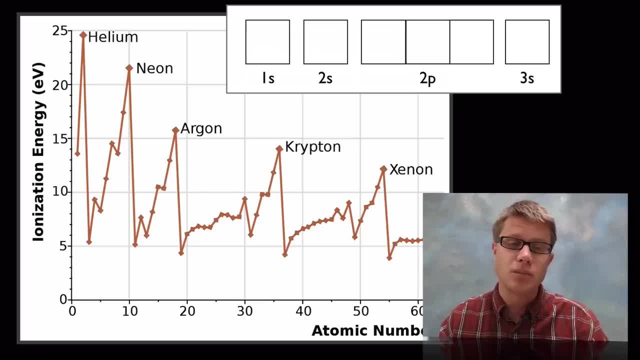 And so let's kind of lay this out for just a second. So a shell is going to be. let's look at the first one. So here we've got hydrogen. So hydrogen is going to be right here And we said it had a high ionization energy And that's because it's really close to that nucleus. 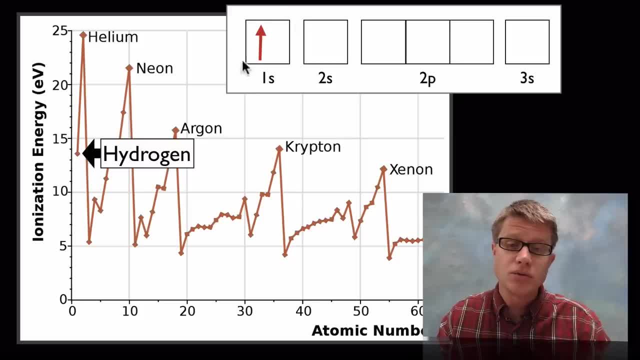 So it's close to the protons inside there, And so what we can do is we can fill out this box. So this is going to be the 1s. We would call it the 1s, And this is going to be the. 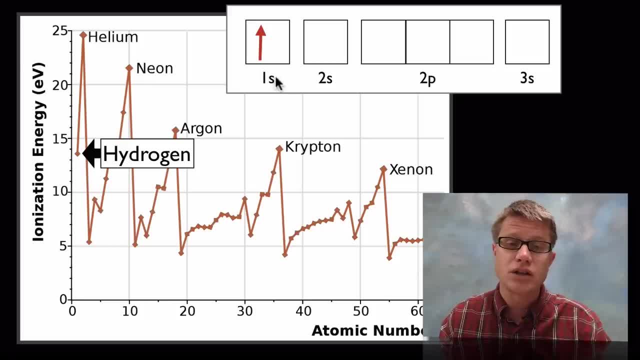 1s shell. But the reason we have boxes here is that it was later discovered that electrons will fill what are called orbitals, And those orbitals can only have two electrons in each one. So let's look at hydrogen. Hydrogen, we said, has an ionization energy, we'll say on. 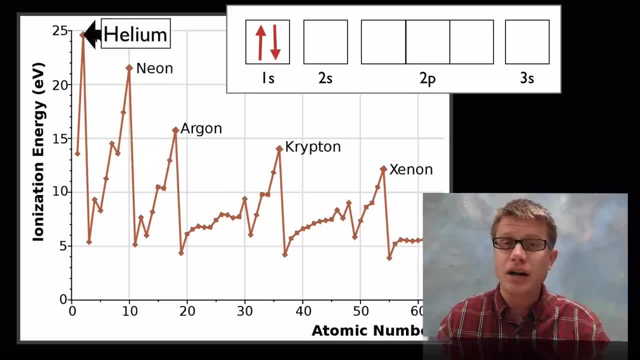 this chart around 12.. If we go to helium, it's going to have a higher ionization energy. Why is that? It's going to be because, remember, we have those protons on the inside that are holding it in. But let's watch what happens when we go to. 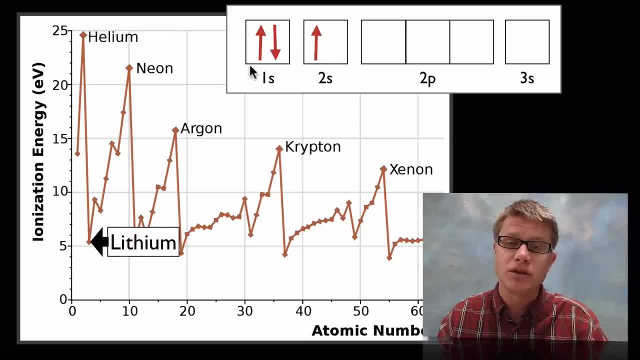 lithium. What's happened is we've gone into this whole next orbital And so there's this shielding effect of this filled orbital here, And so we have much less ionization energy there. Let's watch what happens with beryllium. Well, that kind of makes sense. We're increasing. 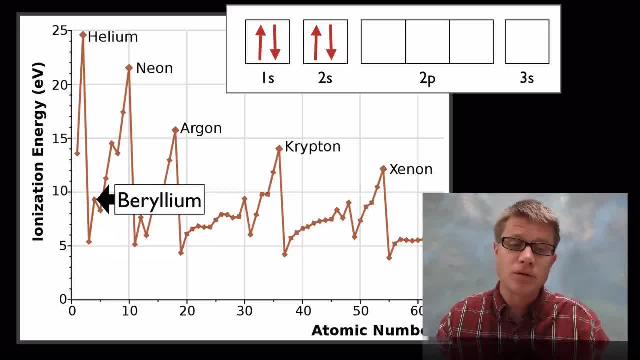 the protons, and so that should go up. But then what happens with the next one? Well, when we go to boron, what's happening is it's actually going into a new orbital, And so it's going into an orbital of the second subshell. And so if we didn't have these orbitals, what? 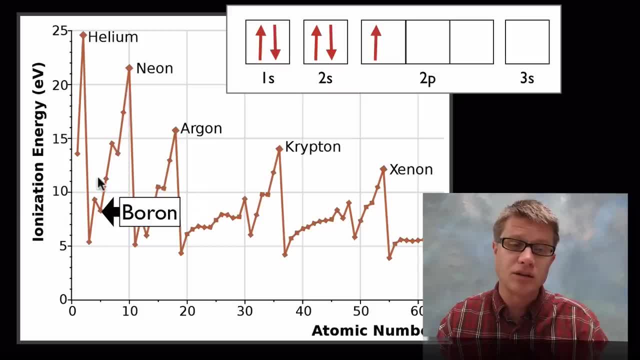 would happen is it would just be a connection between these two. So we're going to have a consistent all the way up to neon. But you can see we kind of have this jag as we move up. If we go to the next one that makes sense. Carbon is going to have more ionization energy. 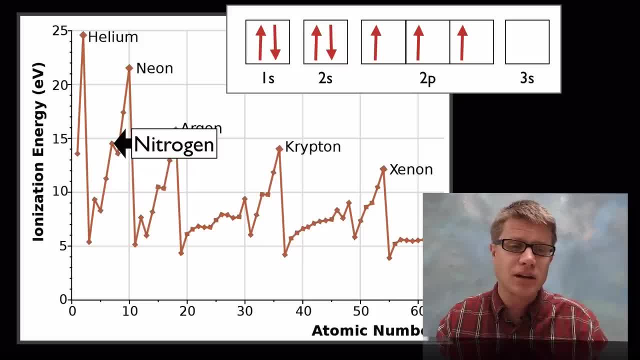 We're adding more protons, Nitrogen same way. But now let's look at this: Why does the ionization energy go here after we leave nitrogen? Well, the reason why is that these electrons are added, And they're added one at a time in each orbital, But they'll have. 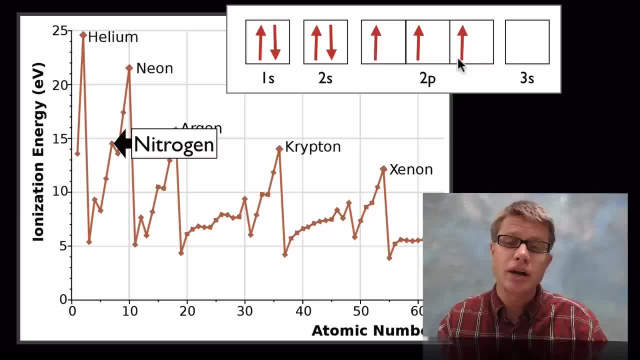 a specific spin, And so you can only have two electrons each way. But what they'll do is they'll fill them, kind of like seats in a bus, And so they're going to all get on one seat per bus, But then when we get more electrons they're going to have to double. 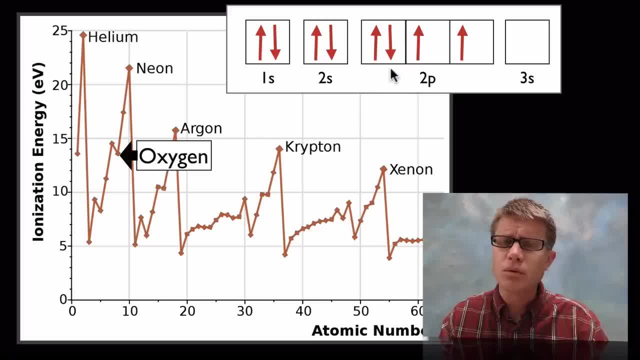 up. And so what happens is, when we go to oxygen, what we're doing is we're making that electron sit in that orbital. It would rather not be there. There's repulsion between those electrons, And so it lowers the ionization energy. We go to fluorine, We go to neon. Once we have. 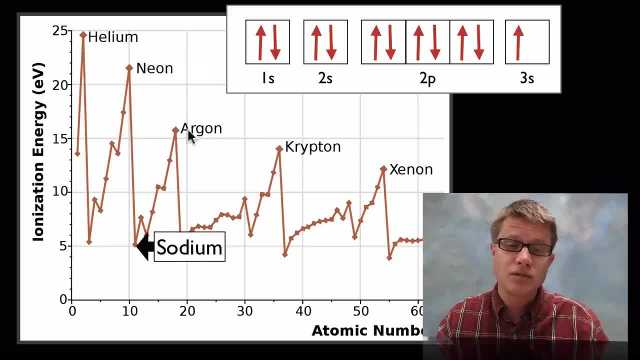 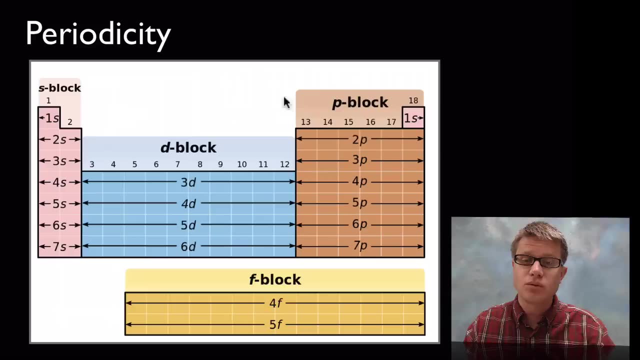 that shield effect, we jump all the way down to sodium again, And so once I really understood what was going on in this chart, then all of these sub shells made sense, And so we're going to have a shell which is going to be the 1,, 2,, 3,, 4,, 5.. But we're also going to 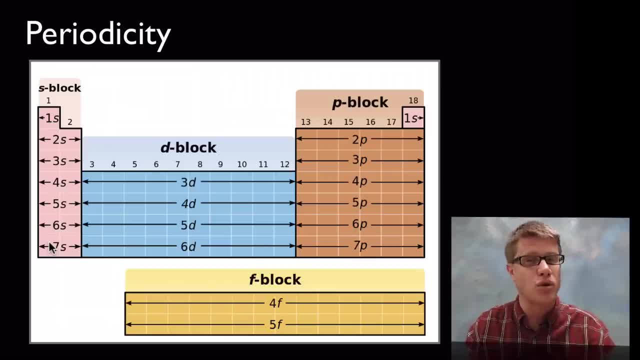 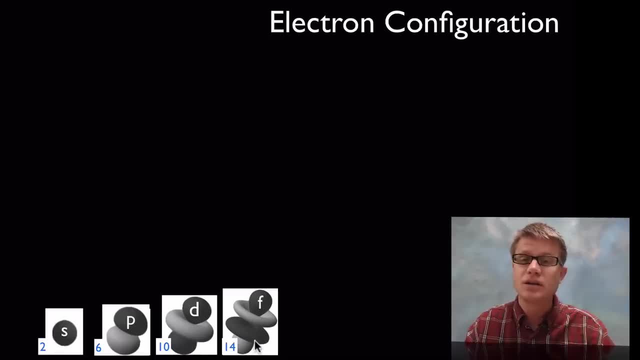 have sub shells which are smaller, And then within each of those we're going to have orbitals, if that makes sense, if we go in size. And so let's get to the electron configuration, And so what we have here are the sp, the d and the f. They come from quantum mechanics. 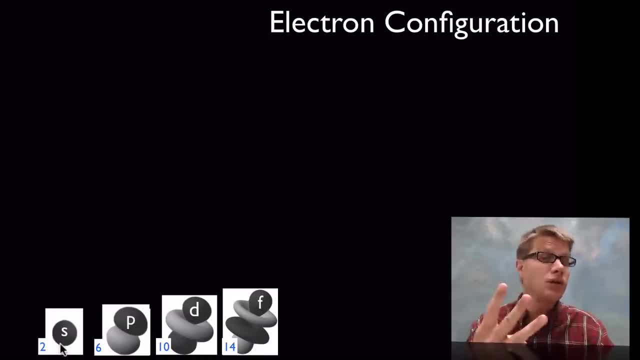 The sp has only one orbital in it, The p has three orbitals, so you could have six electrons. D has five orbitals, so you could have ten electrons, And f is going to have seven orbitals, so you could have fourteen electrons. So if you want to write this out, you could just 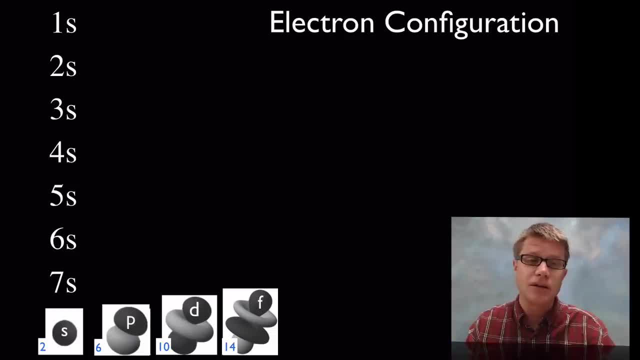 write on a chart, Start with the 1s and just write all the way down to 7.. Then you want to write right to the right of that 1s or 2s. you're going to write the 2. And then you're. 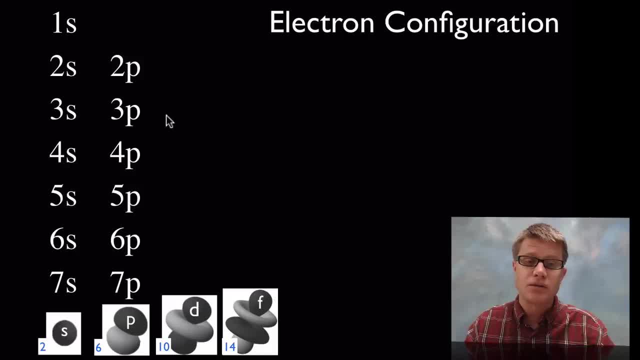 just going to write p's all the way down, And then you go down to the 3.. We'll write a 3 over here, And then you're going to write d's all the way down, And you could go all the way to 7, but we'll never really need that. Then you go to the 4. You write a 4. 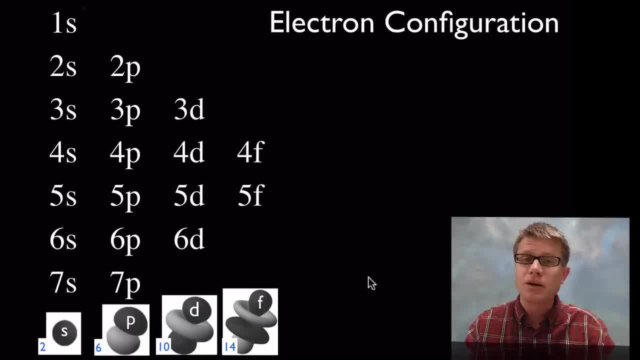 over here And then you write f's all the way down, And so once we have that, we can put diagonal lines in like this, And then we can do the electron configuration for anything. So you wouldn't even need a periodic table, You could just do this and you could figure. 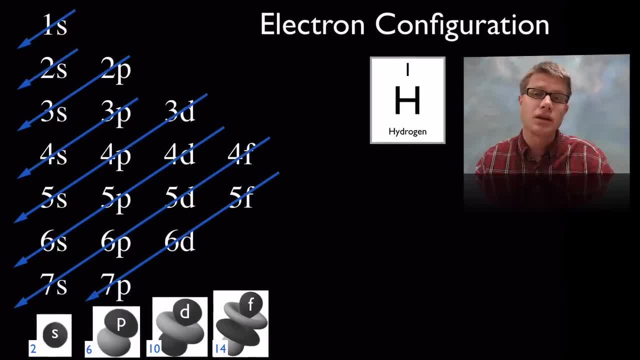 out electron configurations. Let's start with hydrogen. What's going to be the electron configuration of hydrogen? You're simply going to start at the top, And so it's the 1s shell, or orbital, or sub-shell, And so what? we would write it as is 1s, And then we're going to 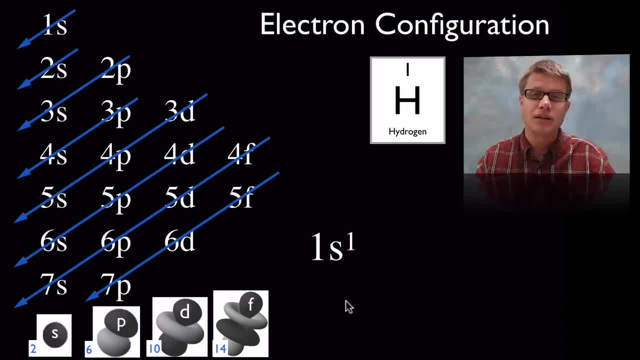 write 1s1. And that 1 represents the 1 electron that we have inside that orbital. If we go to boron, then how are we going to write boron? Well, you're going to start here, go here, go here. Boron is going to be a 1s2, because we can only put 2 electrons in there. We then 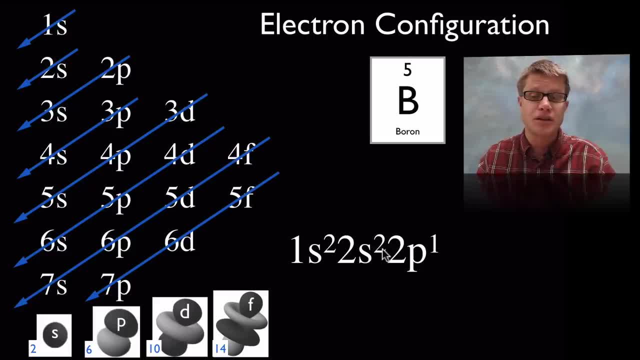 go to the 2s. It's going to be 2s2, because we can only put 2 electrons in that. And then we're going to go to the 2p and we only have 1 electron left, so we're going to put it there. 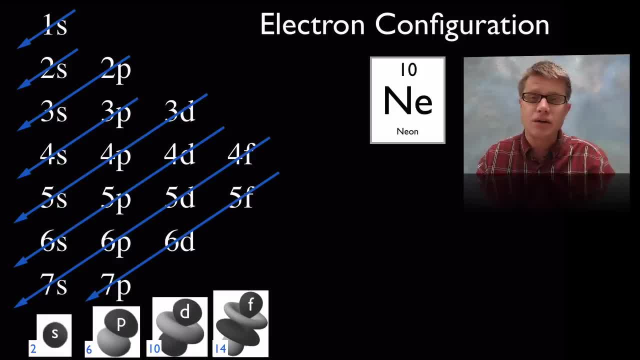 So that would be boron. What about neon? And again, you could pause the video and always try it out. Neon is going to be this, So it's 1s2, 2s2.. 2p, remember, can have 6.. And so we're going. 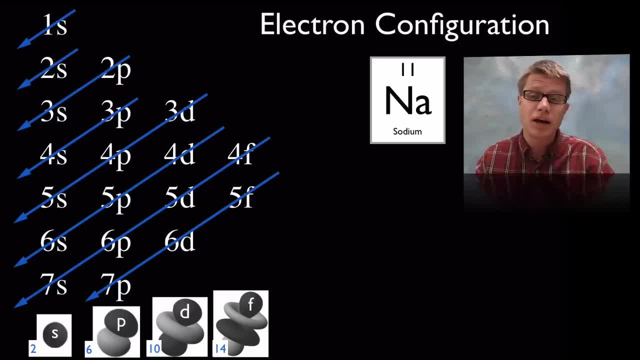 to write 6 there. Let's go to the next one. What about sodium, which is number 11?? We've got 11 electrons. Well, we could write it out like this: 1s2, 2s2, 2p6.. And then the next.